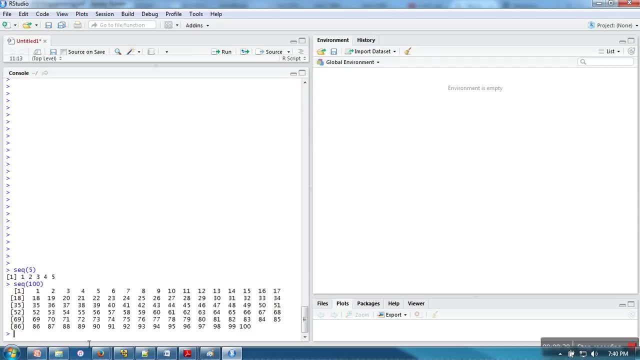 very easy way to generate a number series. now. the thing is that if you want to generate a number series from a specific point, so you can write here like starting point and end point, so it will generate a sequence number from 12 to 90, increased by 1. now, if you want to change this, like instead of increasing, 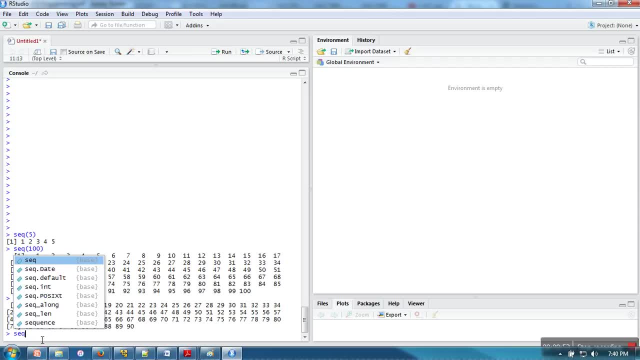 by 1. we want to increase by 0.4. so what I want to do? I want to start from 1.1 and I want to end it at 2 and increase it by 0.1. so then there will be three parameters in this function: starting, ending and by what number you. 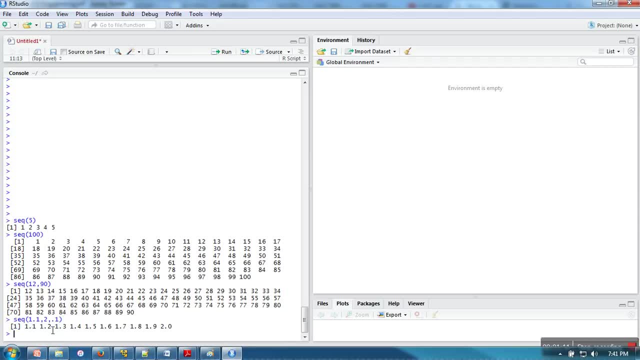 want to increase. so if you can see here 1.1, 1.2, 1.3, so this is very useful function to generate such kind of series. the next one is repetition. so if you want to repeat a number for particular number of time, let's say I want to repeat. 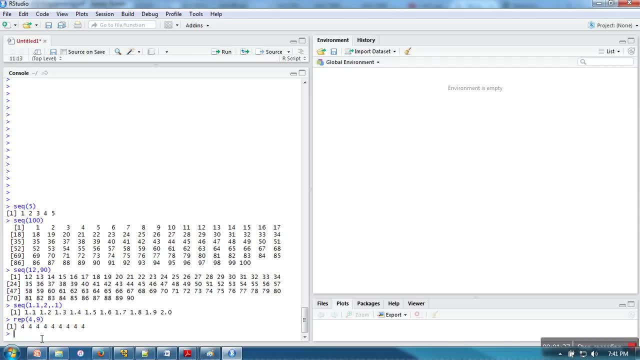 4, 9 times. so it will generate a series: 4, 4, 4, 4, 9 times. so next two are all and any. so for that, first I am going to create a vector and in this vector I am going to take some element. so here what I am going to do, I am going to check whether 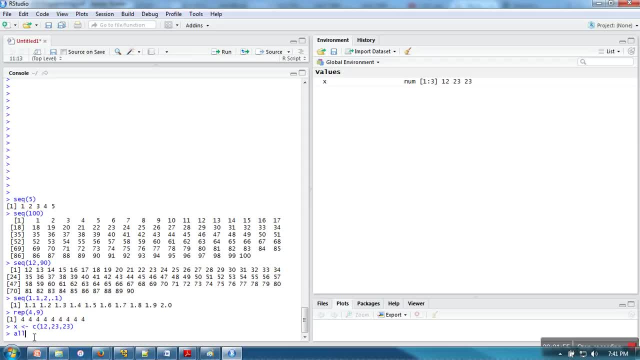 element element in this vector are less than or equal to the number of times as than 20 or not. so when I use any, so what this will do, this condition will be checked against every element of this vector. so 20 greater than 12. so in this, 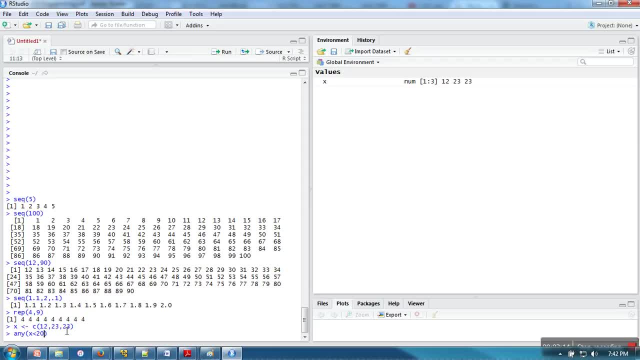 case, true will be returned and in these two cases, false will be returned. so any this function will return true if there is true in the returned value. so if you can see. but in case of all, it will return true in only if every condition resulting true, every condition successfully returned true. so, but in our